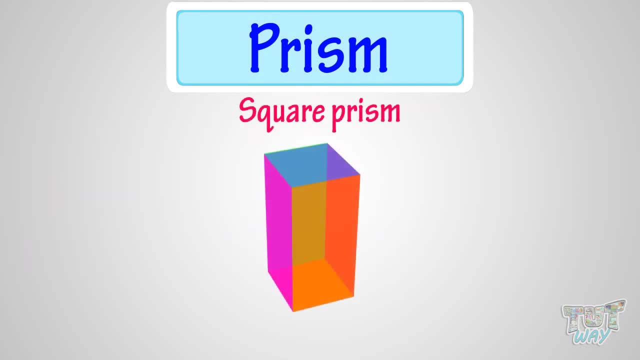 This is a square prism because its top and bottom faces are square in shape and all other faces are rectangular. This is the same as a cuboid, So it has six faces, eight vertices and twelve edges. Now let's learn another type of prism. 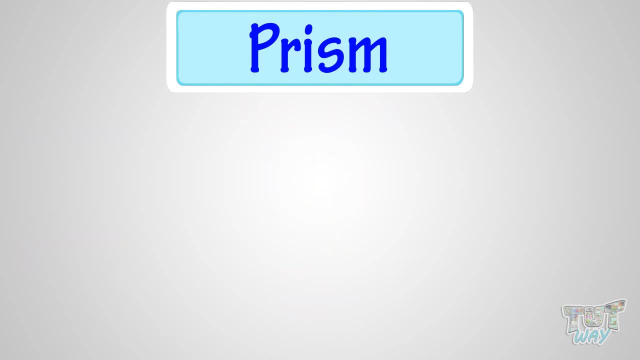 This is a rectangular prism because its top and bottom faces are rectangular and all other faces are rectangular too. This is the same as cuboid shape, So it has six vertices, nine edges and twelve edges. This is the same as a cuboid shape. 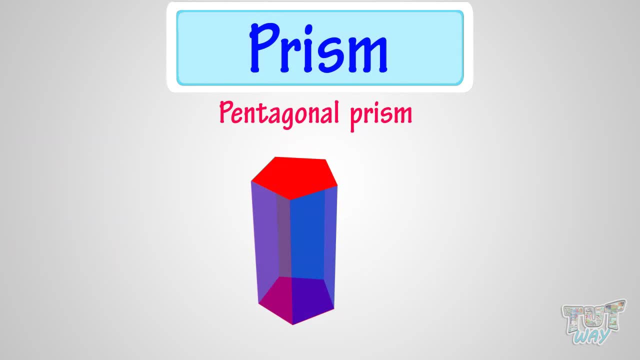 because its top and bottom faces are pentagon in shape and all other faces are rectangular too. So it has six faces, eight vertices and twelve edges. Now let's learn another type of prism. This is a pentagonal prism because its top and bottom faces are pentagon in shape. 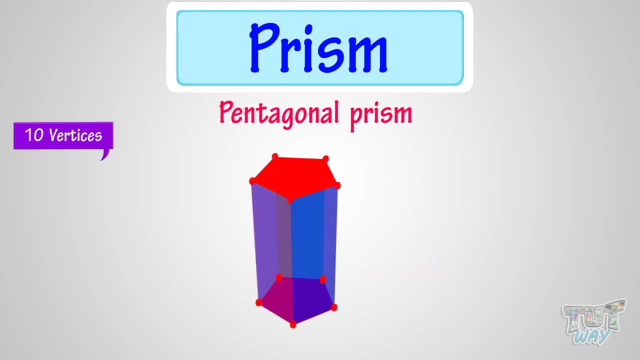 and all other faces are rectangular too. It has 10 vertices, 15 edges and 7 faces. There can be more types too, depending on the shape of its top and bottom faces. Now we will be learning another 3D shape, Pyramid, and its types. 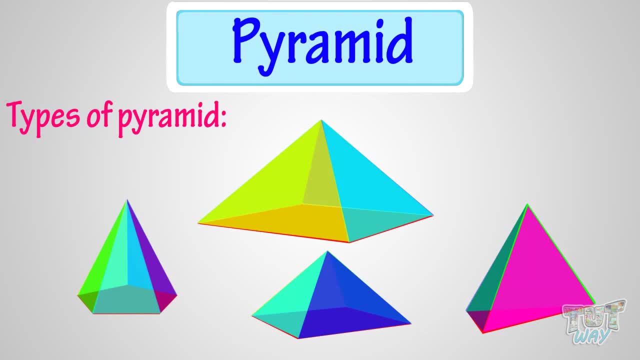 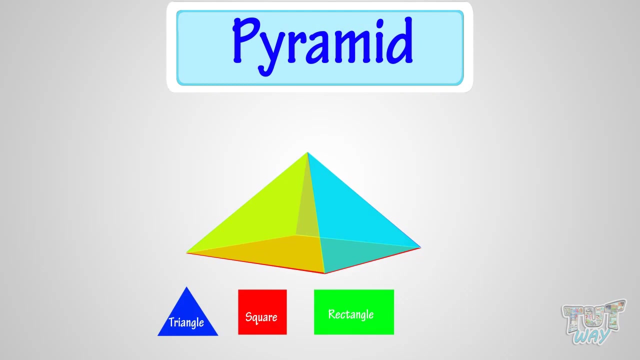 First let's see what is a Pyramid. In simplest words, Pyramid is a 3D shape where it has a single base which can be of any polygon shape like triangle, square, rectangle or pentagon, And all other faces are triangles. 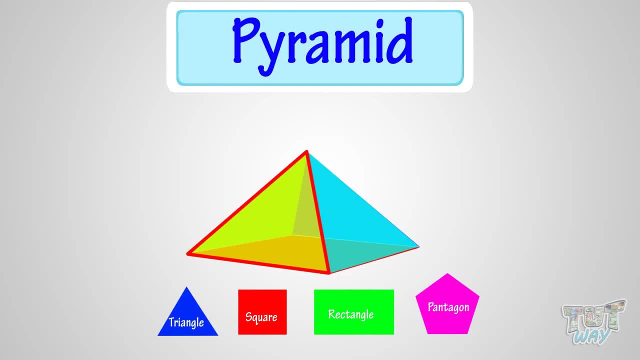 And all other faces are triangle in shape that converge to a single point at the top, which is called its apex. I repeat, Pyramid has a single base, which can be of any polygon shape, like triangle, square, rectangle, And all other faces are triangle in shape that converge to a single point at the top, which is called its apex. 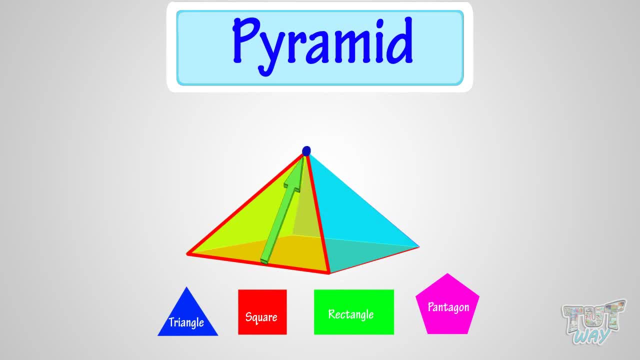 And all other faces are triangle in shape that converge to a single point at the top, which is called its apex. Most common Pyramids are with triangle and square bases. Here are examples. This is a triangular Pyramid because its base is a triangle. 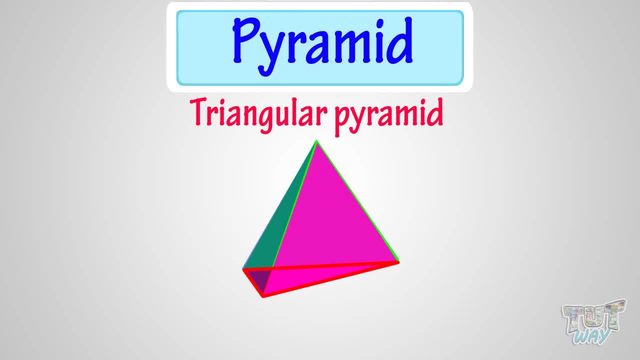 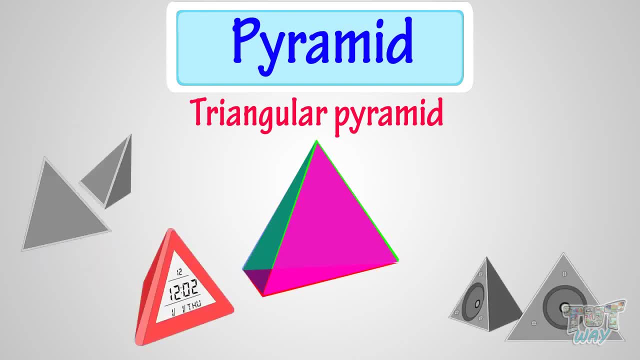 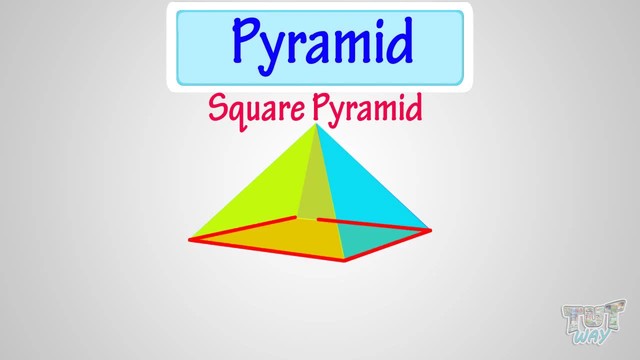 These are common things of this shape. This is a square Pyramid because its base is a square And all other faces are triangle And converge to a single point And all other faces are triangles and converge to a single point. It has five vertices, eight edges and five faces. 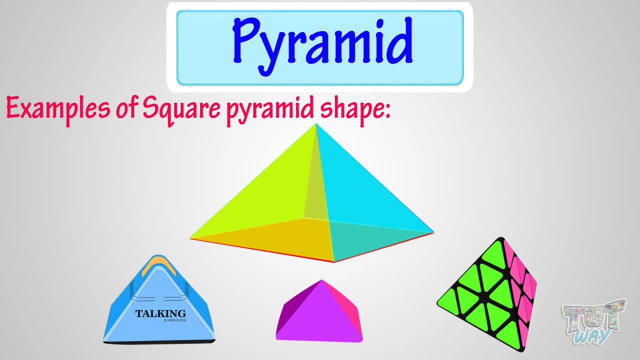 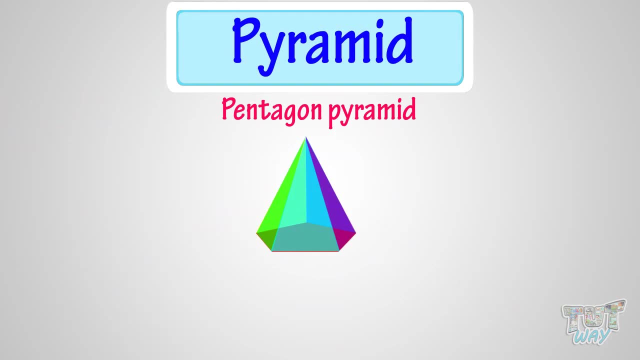 These are some common things of this shape. Now, this is a pentagon pyramid Because its base is a pentagon and all other faces are triangle and converge to a single point. It has six vertices, ten edges and has six faces. 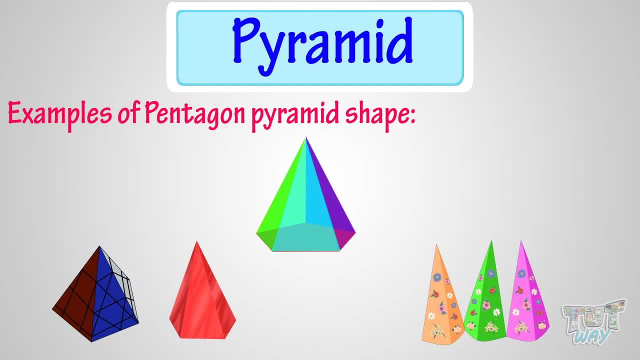 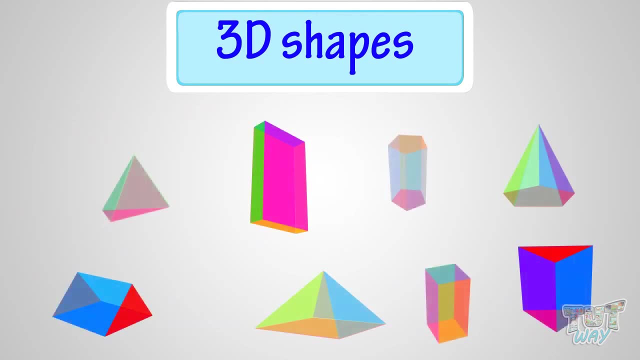 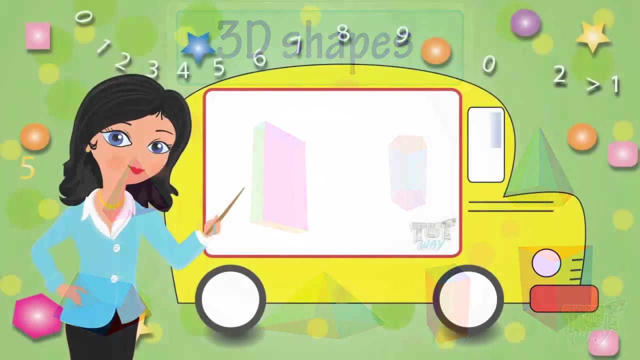 These are some common things of this shape. Okay, kids, Today we learned various interesting 3D shapes. Hope you enjoyed learning, as I did while teaching. Now you may go ahead and take a quiz to learn more. Bye-bye.